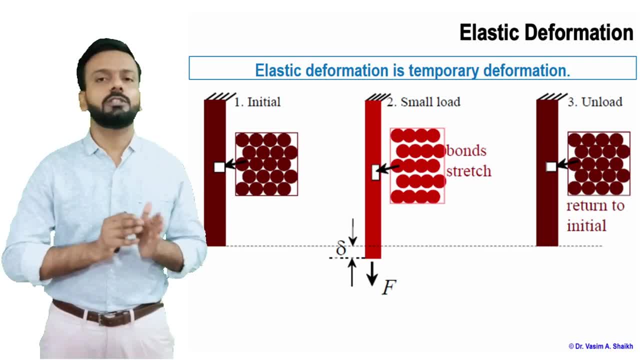 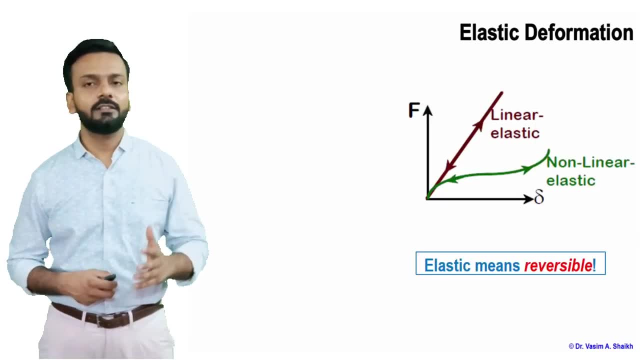 change the diameter and then it will go back to the original shape as we release the load or remove the load. so that is elastic deformation. and the elastic deformation can be of two types here. it can be either linear elastic or it can be a non-linear elastic. the end result is the elastic. 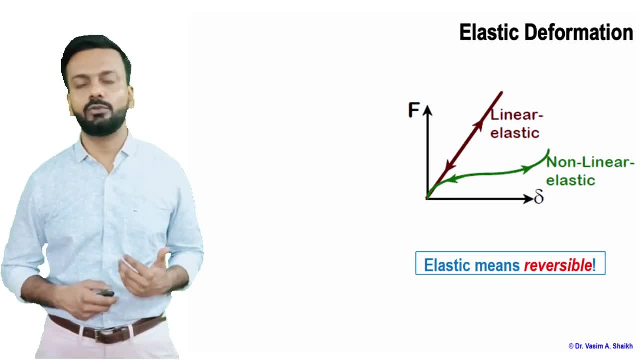 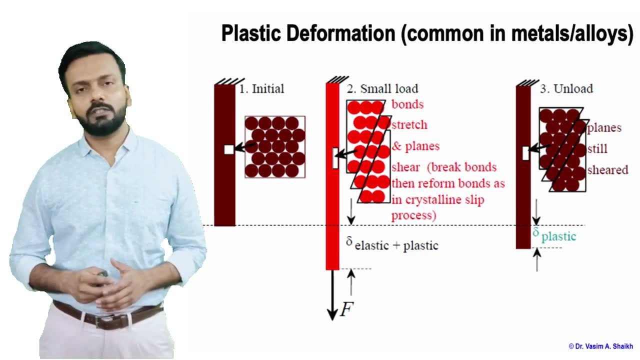 means it is reversible and it will revert back to the original shape. now let us see what is plastic deformation. so the same scenario: you are applying the load, the bonds of the material are stretching, but here you are applying the load in such a manner, you are increasing the load in such a 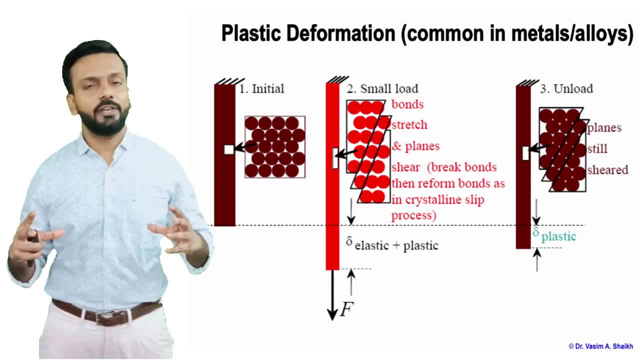 manner that the length is increasing. and when you release the load, when you remove the load, some part of the material is recovered in the elastic deformation. but there is a permanent deformation and the material when it tries to go back to the original shape, it cannot go back to the original shape because some of the bonds of the material are broken. so the bonds are. 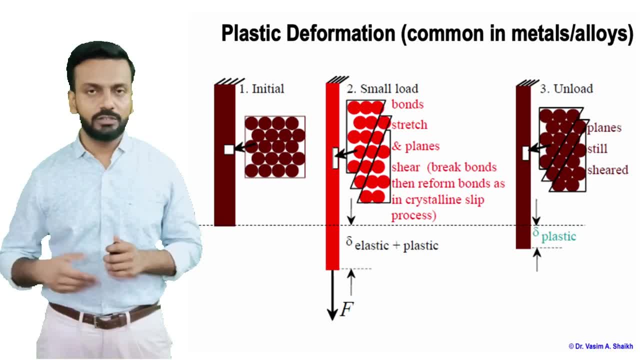 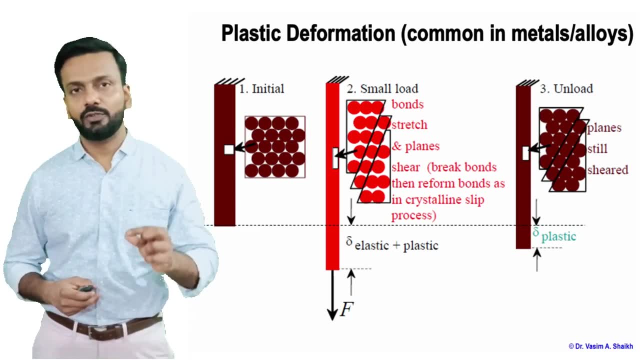 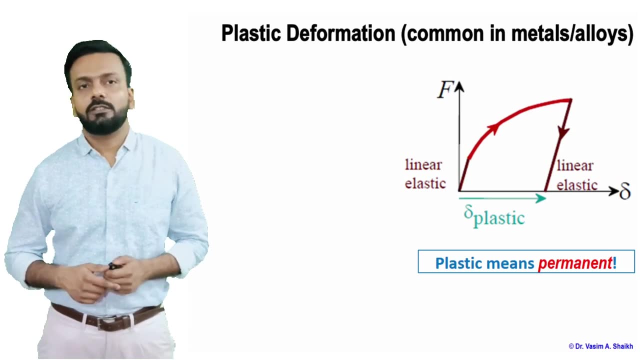 broken and the material cannot go back to the original shape. there is some permanent damage that has happened to the material and that is called as a plastic deformation. this is very common in metals and alloys. so here we see the range or the load and the deflection of the plastic deformation. so you are applying the load. 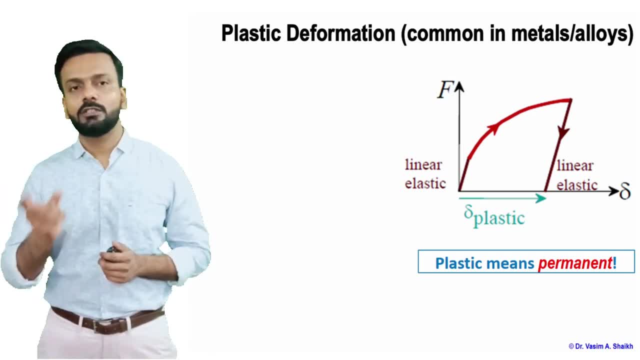 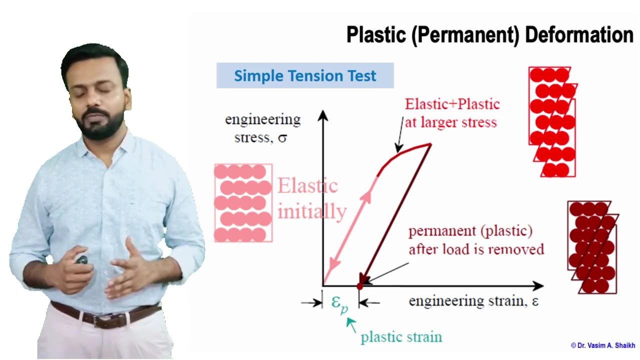 it has reached to a point and then, when you release the load, some sort of deflection or change in shape, which is plastic in nature, is there, and plastic means nothing but permanent deformation. now, this is a very normal and simple scenario of the simple tensile testing. and here 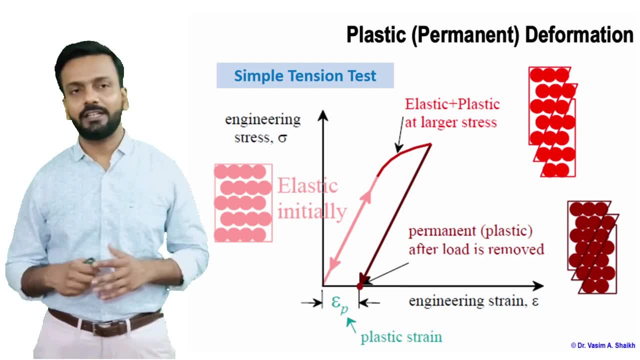 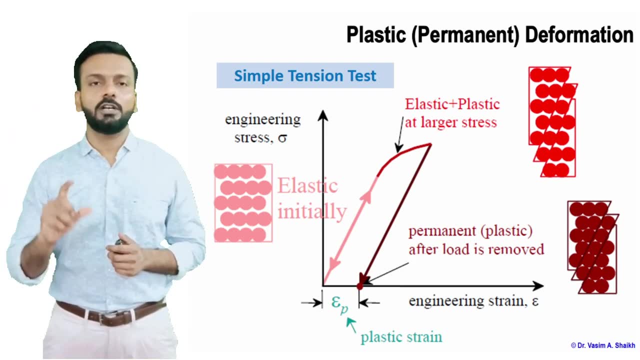 you can see the plastic deformation. how does that happen? you have the deformation of the plastic, and How does that happen? You have a stress strain diagram. You are applying the load, You are increasing the load, The load reaches to a yield point, The material starts to yield and then, when you release the load, the material goes back to some of the original position it takes and then it will have some sort of deflection, which is permanent deflection, and the material will go through all this. 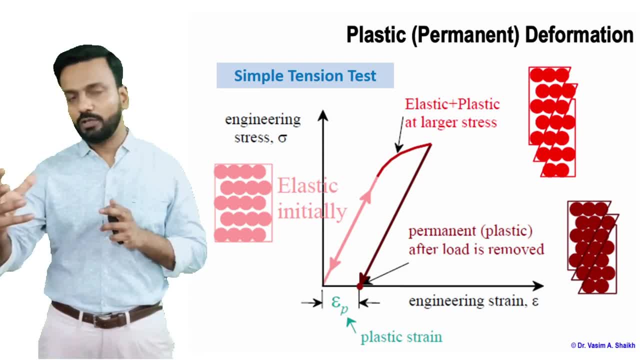 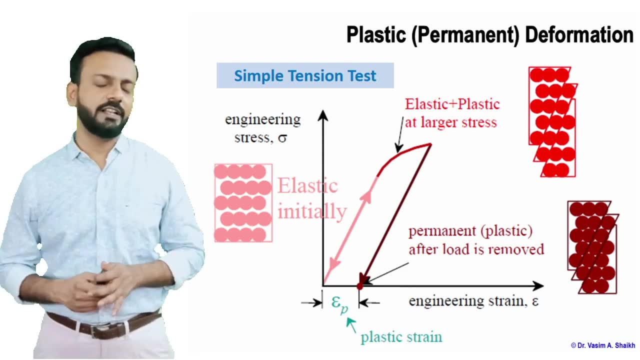 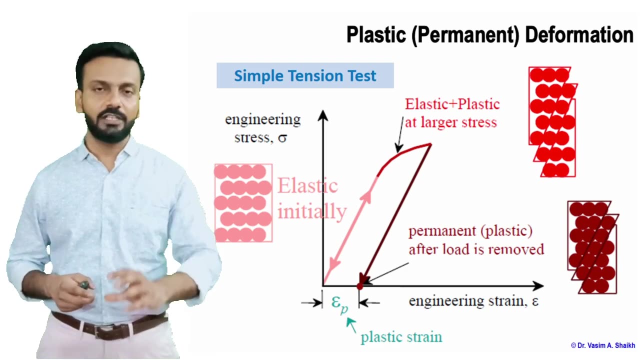 And then you have the bond which is shown. Then some bonds are broken and then when you try to release the load it will go back not to the original shape, but some elastic strain is recovered. The elasticity is recovered and then some permanent damage has happened to the material. It will have some sort of change in length. That change in length will be little bit more than the original length. 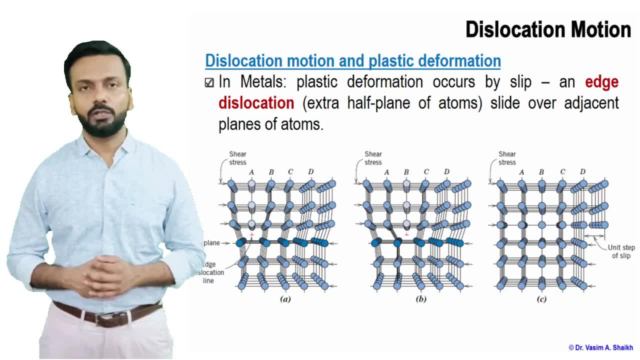 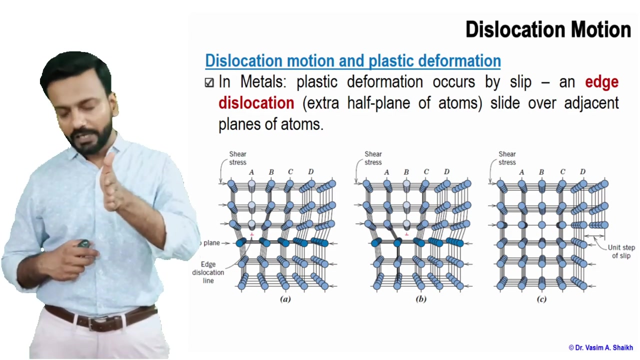 So let us move on further and see what is the dislocation motion Now. how does that happen? So how does this plastic deformation and slip mechanism, all this fit in with the dislocation motion? So this is an edge dislocation which we are seeing here. Extra half plane of atom is there and then this is there on a slip plane and then edge dislocation will try to move on the slip plane when you are applying the load from either side, Then the dislocation will go on moving from plane to plane and then it will try to break the bonds and then it will move further and finally it will move on and a yield point. 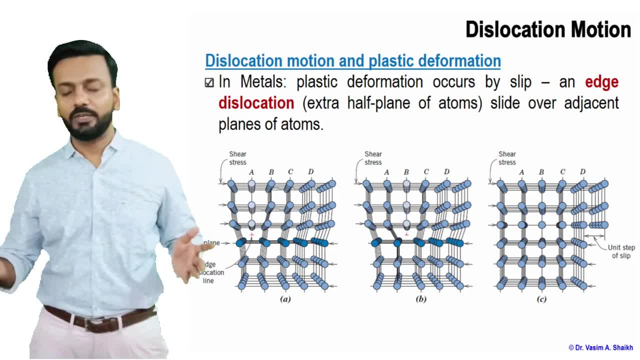 So this is the unit step of dislocation- will remain. that is nothing but a Burgers vector, which we have seen in the earlier video. So this is how the dislocation tries to move and because of this dislocation, we have the plastic deformation that is taking place. The material is trying to deform, change the shape, change the size, and then this is nothing but at a microscopic level. this is happening because of the dislocation motion of the material. 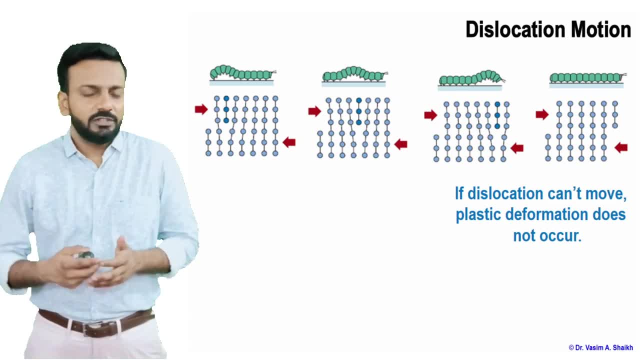 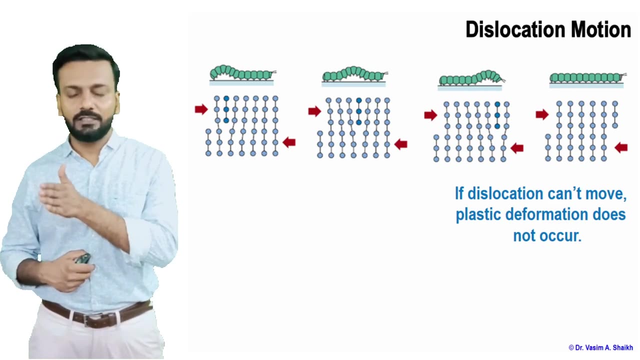 So it can be an analogy which we are seeing here, like a worm: How does this dislocation move, How the worm is moving, and then it is going, and then how it is moving further. So this is the analogy of the worm which we are giving to edge dislocation and that how this edge dislocation is moving, as in the worms are moving further, and then finally the material is deforming plastically. 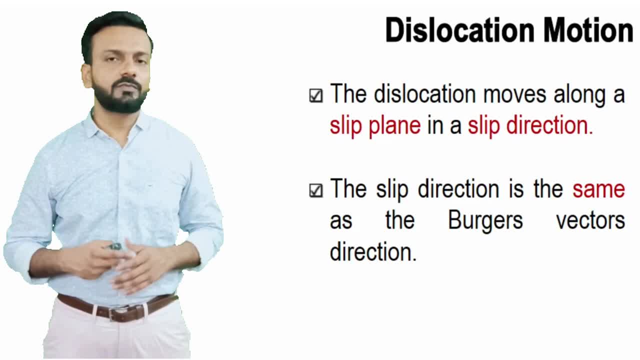 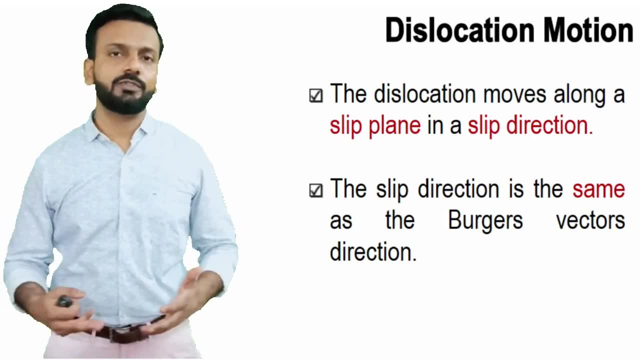 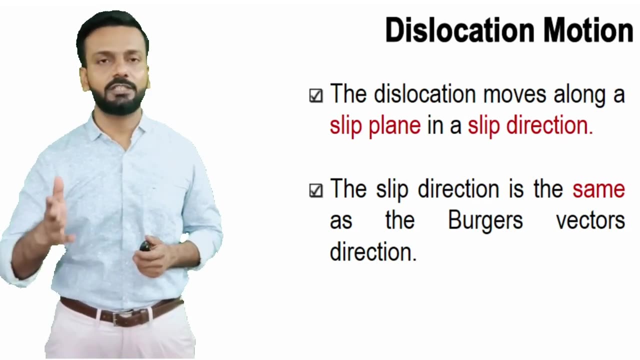 Dislocation motion. The dislocation motion or the movement of the dislocation along a slip plane in a slip direction. So the dislocation moves along slip plane and in the slip direction. so the slip direction is the same as the burger's vector direction, so the slip plane, so the dislocation will move along a slip plane and in a slip. 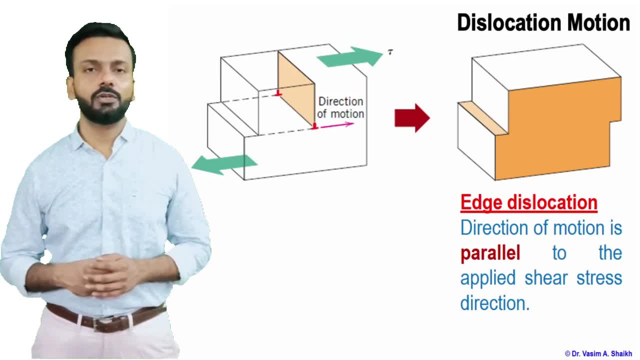 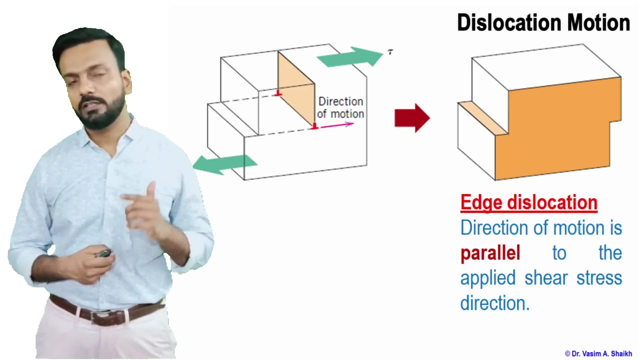 direction. so now let us see a scenario of edge dislocation. we will take that how this can be applied to edge dislocation. so the direction of the motion is parallel to the applied shear stress. so here you see that the arrows in blue color, the load is applied and then the dislocation is moving. 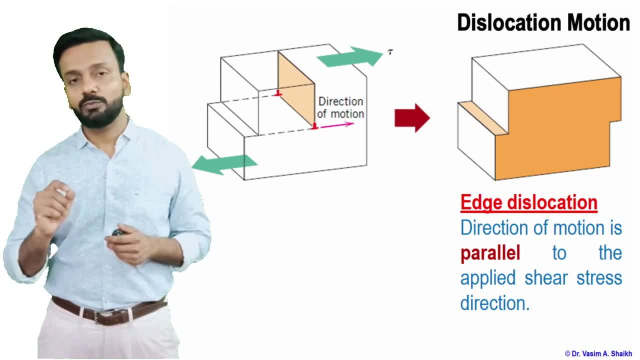 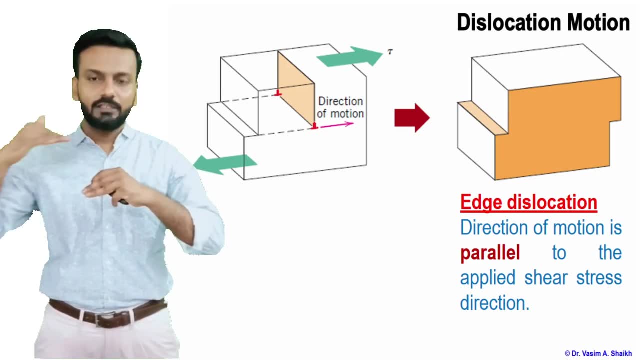 as in shown by the arrow, and that dislocation is moving parallel to the applied shear stress. so the shear stress is applied in this direction. it is moving and the dislocation is also moving in this direction. so the dislocation is moving parallel to the applied shear stress. 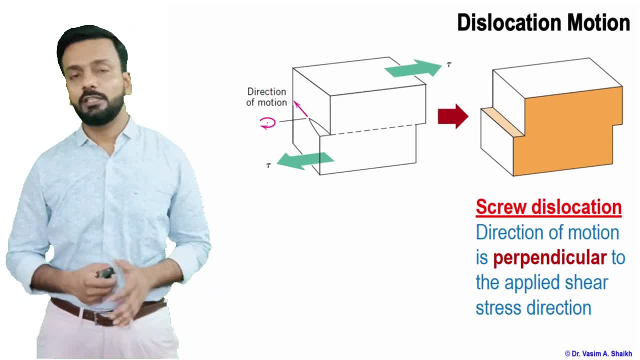 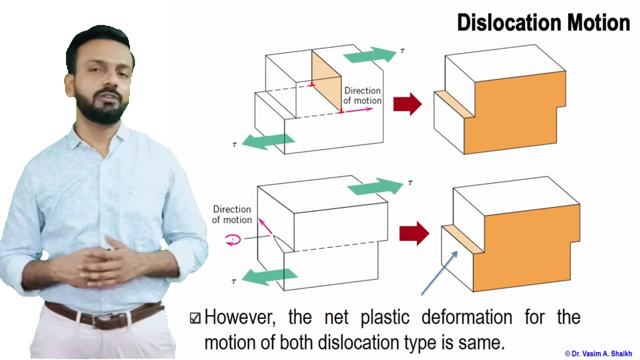 now let us see a scenario of a screw dislocation. here you can see the dislocation is perpendicular to the applied shear stress. So that is the difference between the motion of dislocation, between edge and screw dislocation. But finally, what will happen? Finally, the plastic. 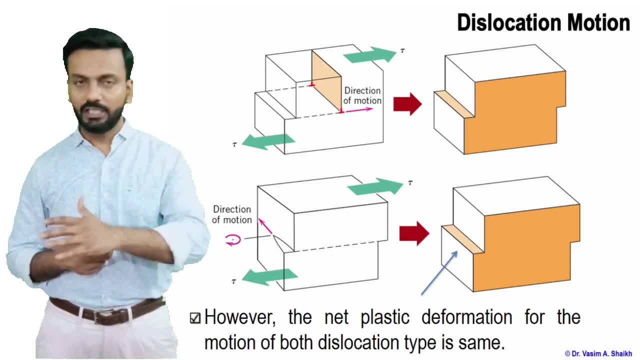 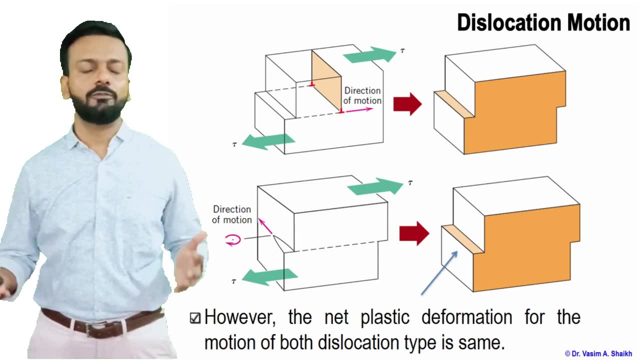 deformation motion, for both is same. The unit step which they are producing, the Burgess vector is the same. Whether it is an edge dislocation or a screw dislocation, the final output or the net dislocation which is happening, the net vector which is happening in the end is the same. So 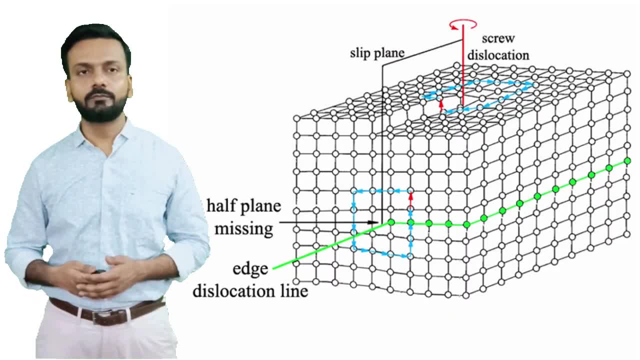 that is not different. So again, one more image where we can see the edge and screw dislocation. The extra plane of atom is inserted, which is shown in green color, and then the dislocation loop of the screw dislocation is shown in blue color. and this is how, But the end result which? 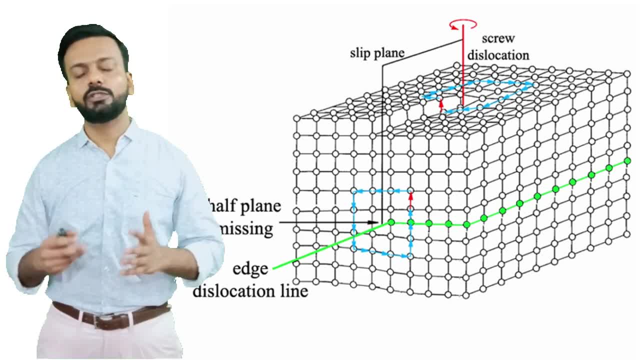 we want to show here is that the Burgess vector is Incorporated. So that means Burgess vector is Incorporated. So that means Burgess vector is Incorporated. So that means Burgess vector is for both is same, and that will not vary either. it is edge or screw dislocation. 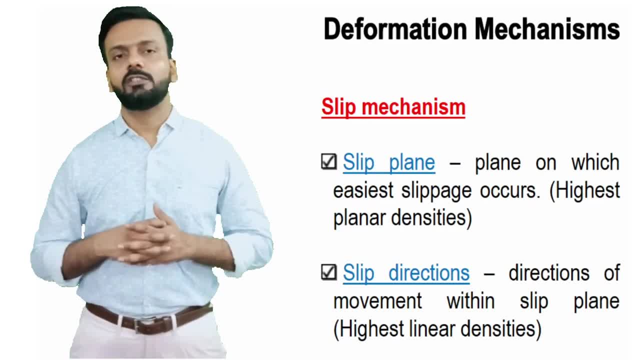 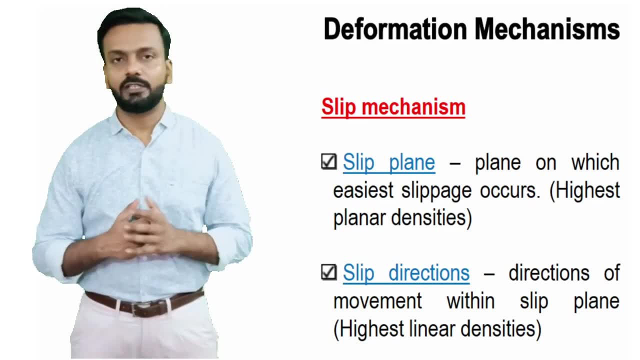 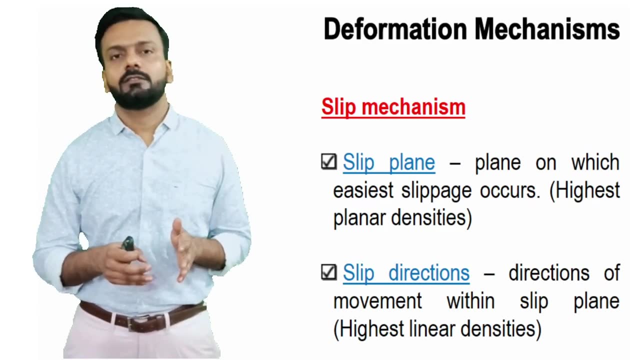 so now let us see what is the deformation mechanism, how the deformation forms and what happens actually in the material when the material is trying to deform itself. so this is nothing, but this is a slip mechanism. so a slip mechanism is consisting of a slip plane and a slip direction. so what is a slip? 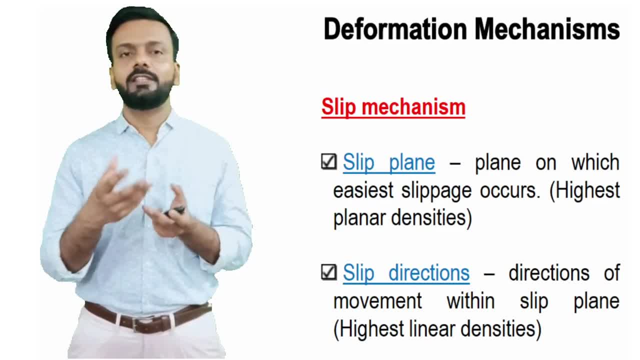 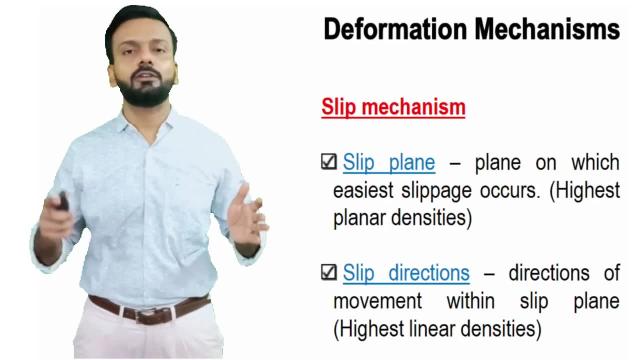 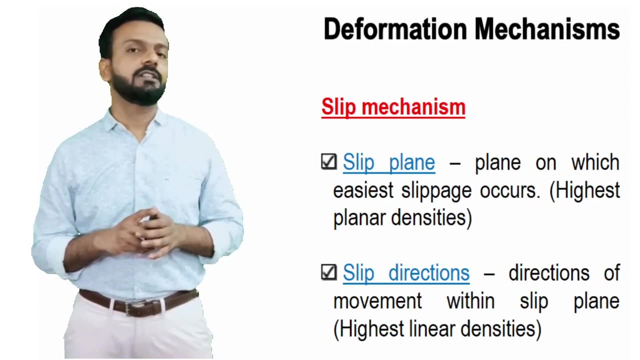 plane, a slip plane, is nothing but a plane where there is a highest planar density. that means atomic density on that particular plane is the highest in that particular structure. similarly, when we see slip direction, that particular direction in that structure, that direction has the highest linear density. 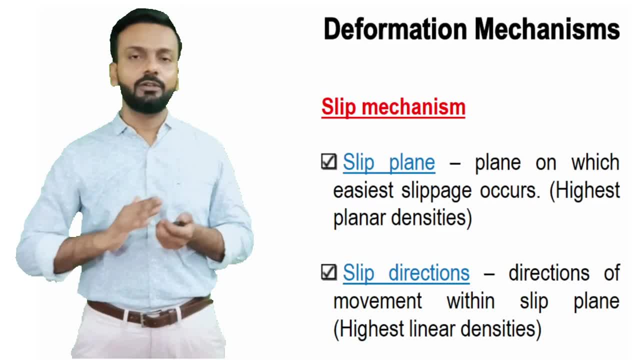 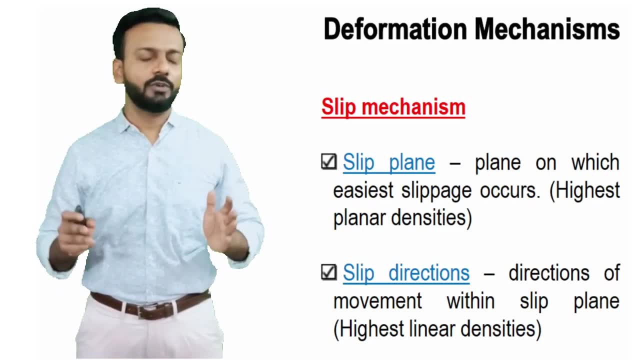 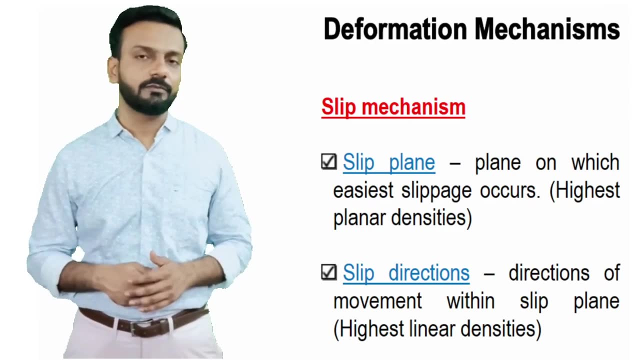 that means most number of atoms are there in that particular direction. it can be anything in terms of FCC or BCC. we will see further. what are these? so, just for remembering, we can say here that slip mechanism consists of a slip plane and a slip direction. all right, so let us move on further. so here we are. 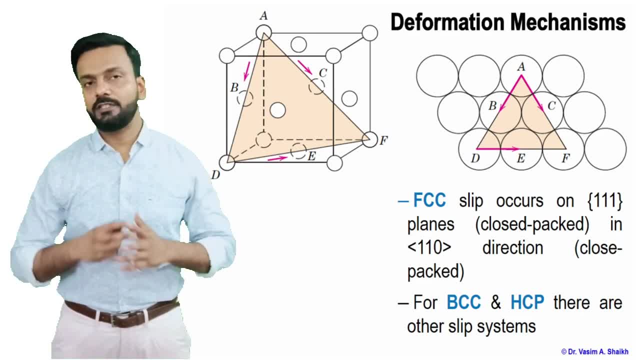 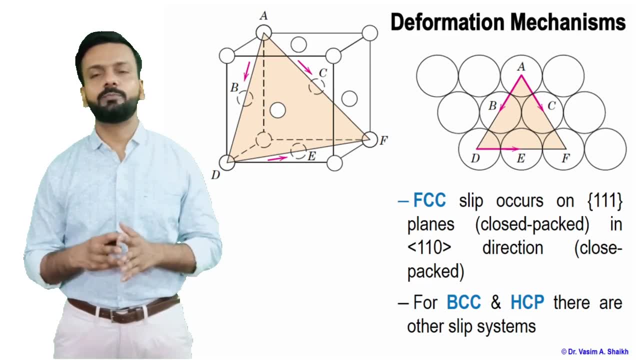 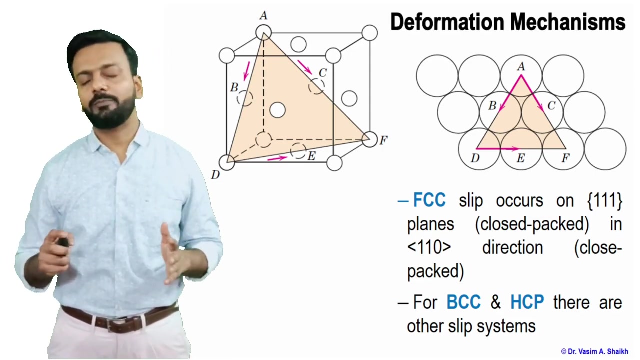 seeing an FCC material and FCC unit cell. so in an FCC the one one, one plane or the one one, one family of plane is the close pack plane, means the one one, one plane has the highest atomic density. okay, and here we can see that the close pack direction is 110. so one one one is a close pack Plane and 110. 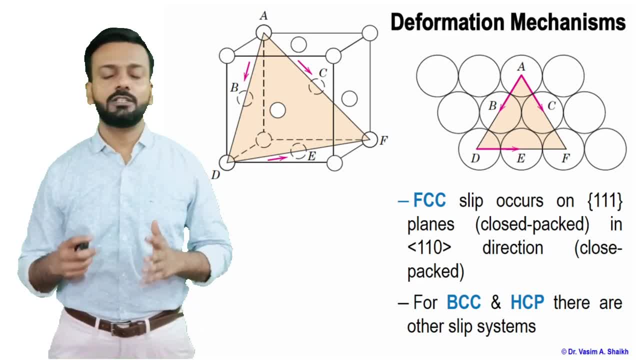 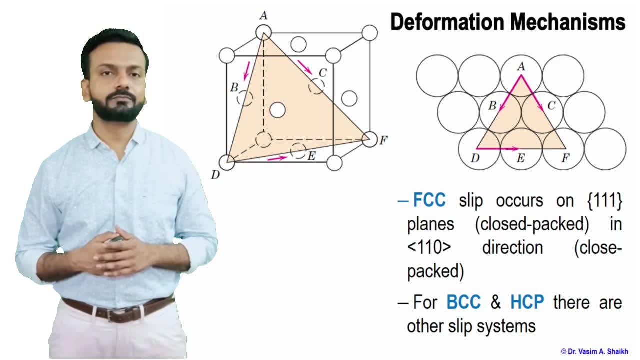 direction or the one one zero family of Direction is the closed pack direction, and for BCC and HCP there are other similar close pack playing and close pack direction. so now let us take FCC, FCC as a close pack, plain family of plane, that is one, one one. and the close pack direction is one one, zero direction. 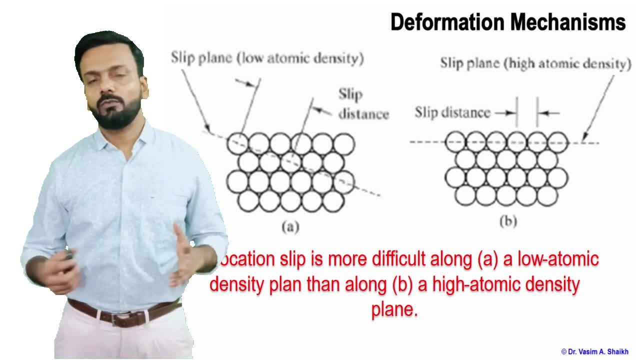 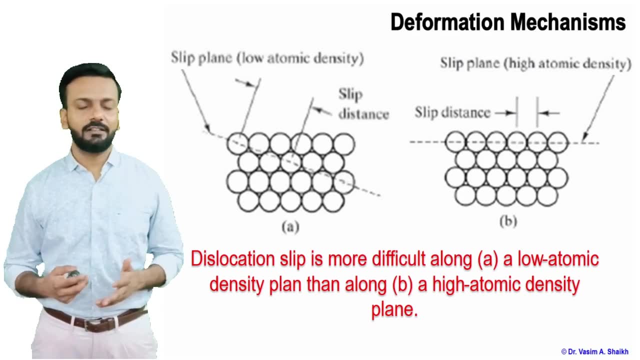 So why the dislocation will happen along the slip plane and in that particular direction. that scenario will cover here. So imagine a slip plane with low atomic density and a slip plane with higher atomic density. So here on the image which is there on the left hand side, you are seeing that if a atom 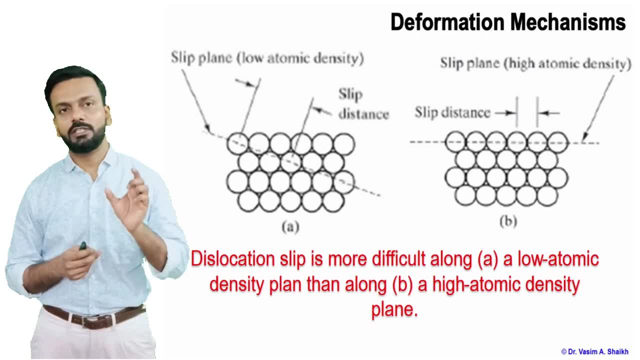 wants to jump from that position, the distance, the slip distance, is very high So it will take a longer amount of stress for jumping from that particular location to the other one and it has to cross a very longer distance. But in the other plane, on the right hand side, you can see that the slip distance for the 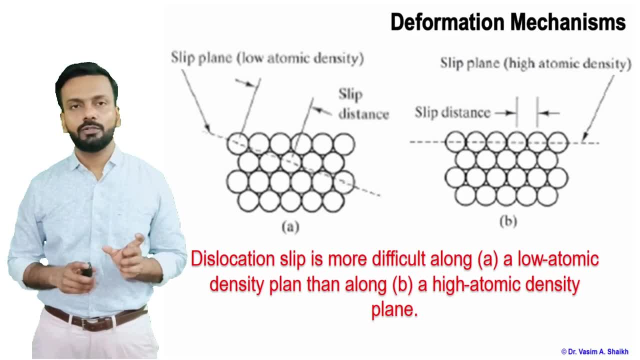 material or the atom to jump over is very small. So when the load applied needed for the material to jump or for the atom to jump over the jump from one place to another is low, it will take that particular route for going from that position to the another position. 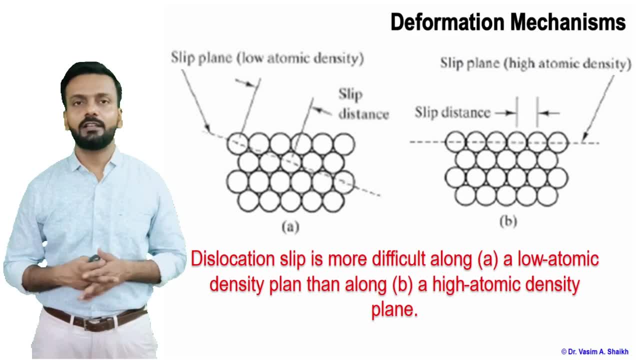 So basically that is what is happening When you have a higher atomic density plane. the atoms are very closely tied together and it needs very minimum amount of stress for jumping and for deforming. So atoms are jumping from one place to another is nothing, but they are helping the material. 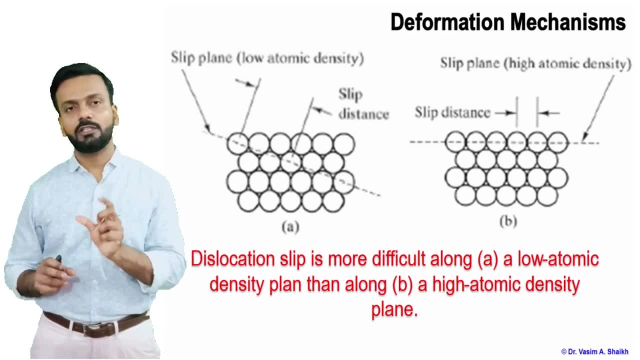 to deform. Okay, So if the slip distance is smaller the material can easily deform. So dislocation slip is more difficult along the figure A, which has the lowest atomic density plane, and the slip can easily happen on the higher atomic density plane which is there. 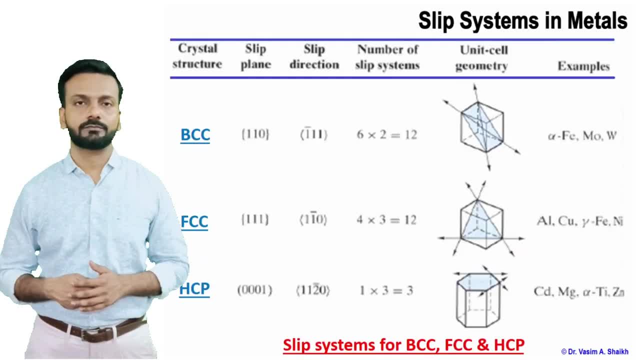 on the right hand side, figure B, So slip systems in metal. So what are the slip systems for BCC, FCC and HCP? So in BCC, Let us see, Let us start with BCC. So in the BCC the slip plane is 1, 1, 0 and that is the family of slip plane where you 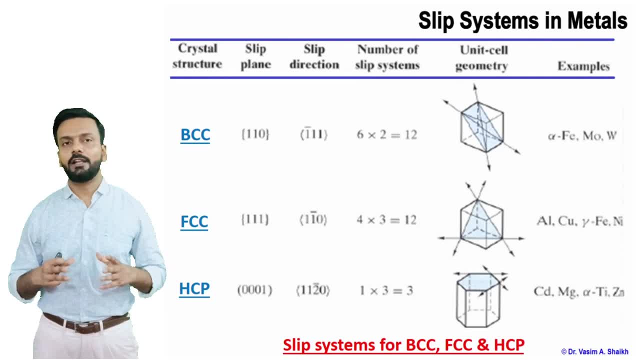 have highest atomic density and the slip direction which has the highest linear density is 1 1, 1 direction. So if we imagine a BCC material, the 1, 1, 0 family of plane has six unique type of planes And the 1 1, 1 direction, the family of 1, 1, 1 direction. in each plane we have two unique 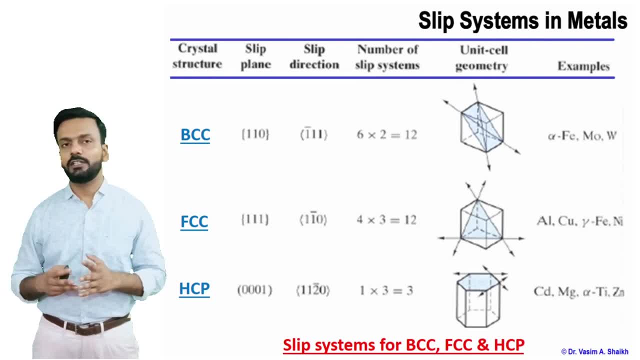 direction. So six unique planes, two unique direction. number of slip systems, or number of ways by which the material can deform, comes out to be 12.. Alpha, ion and tungsten are such material which have BCC structure, and there are 12 unique. 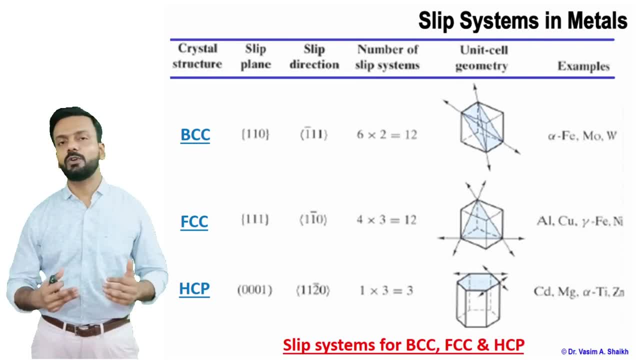 ways by which the material can deform. Now let us move on to FCC. Now let us move on to FCC. Now let us move on to FCC. FCC, the slip plane, is nothing but 1 1, 1 plane. So in FCC, the 1 1, 1 family of plane is the closely packed plane and the 1 1, 0 direction. 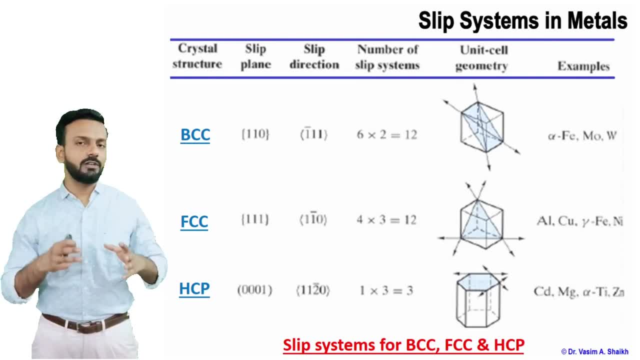 is the closely packed direction. So 1, 1, 1 family of plane. there are four types of such unique planes and there are three unique 1, 1, 0 direction in an FCC material and total comes out to be 4 into 3, that is. 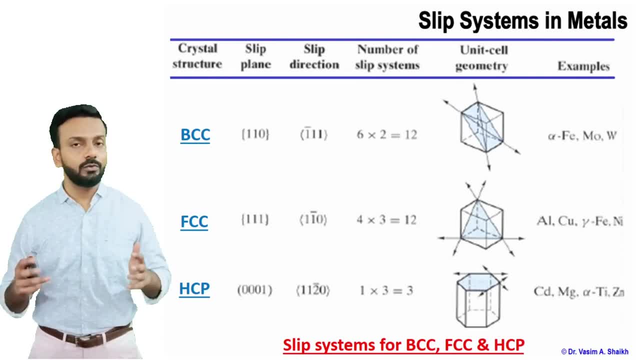 12. So again, in an FCC material you have 12 unique ways or 12 different ways by which the material can deform itself. So more number of such planes, more number of such combinations of slip plane and slip direction. that means the material can deform easily. 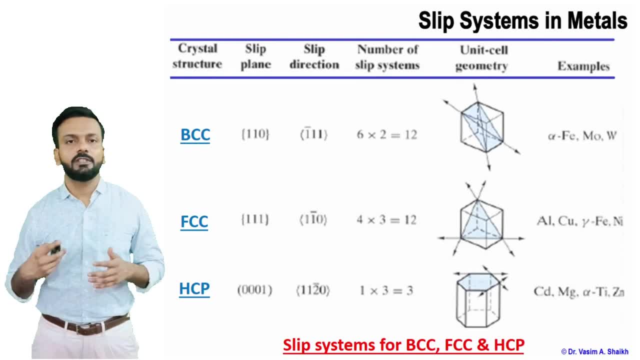 And material like aluminum, gamma ion, copper- all these are nothing but FCC material. and then you can deform this material by 12 different ways. Now let us move on to FCC. So, again, in an FCC material, you have 12 unique ways, or 12 different ways, by which the material 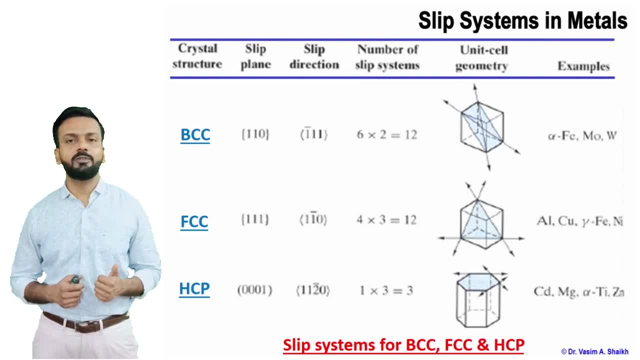 can deform itself. Now let us move on to HCP. In an HCP material, the Basal plane or the 0, 0, 0 plane is the plane which is closely packed and 1, 1, 0 direction is the closely packed direction. 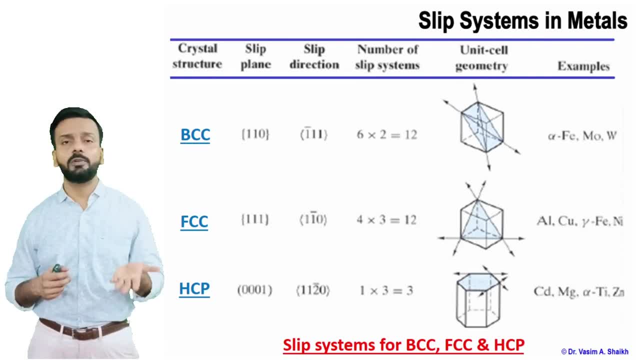 So in an HCP the Basal plane is the only plane which is close packed plane. So it is one unique plane and there are three unique 1, 1, 0 directions, So 3 into 1, there are three unique ways in which the HCP material can deform. 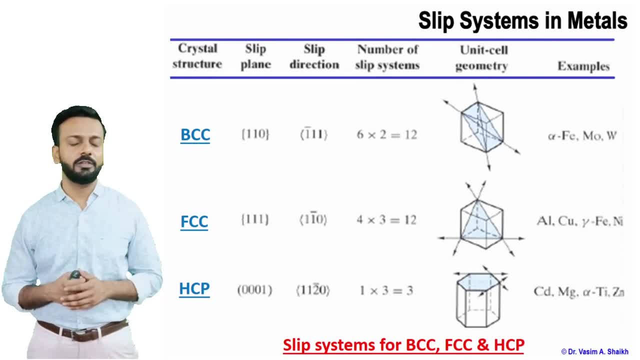 So you can compare FCC's, FCC, BCC and HCP. so we can say that FCC and BCC material can easily deform because there are 12 unique ways by which the material can deform and HCP only has three unique ways by which the material can deform. so HCP will need. 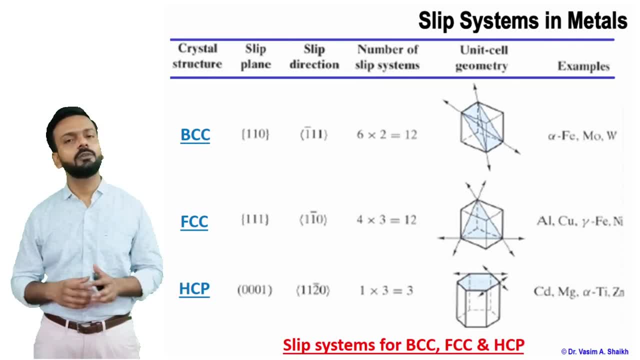 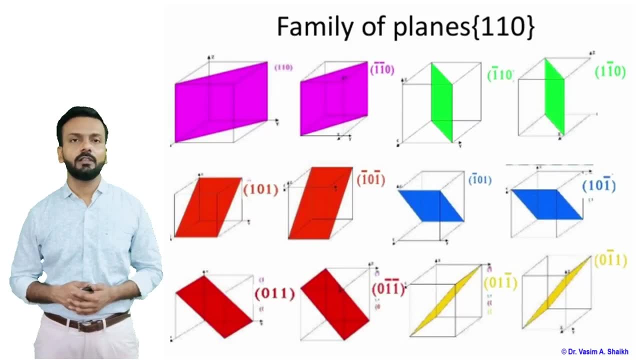 more load, more stress for the material to deform, and HCP and BCC and HCC will take lesser load and they can easily deform. now, here again we can see one more example where we see family of planes of 1, 1, 0 direction. so all the 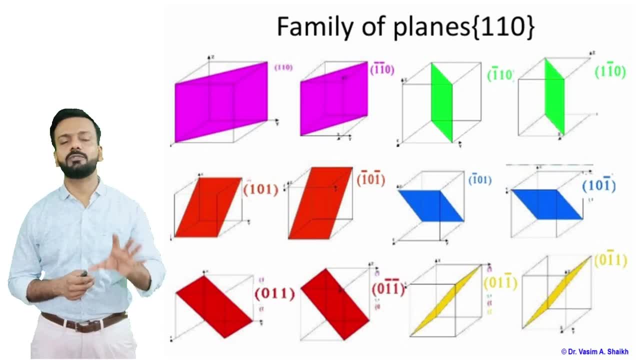 color coding is given that all there are six unique types of planes and this six unique types of plane are nothing but a family of 1 1: 0 plane, and a BCC material has six such type of unique planes and two unique direction on each of these.